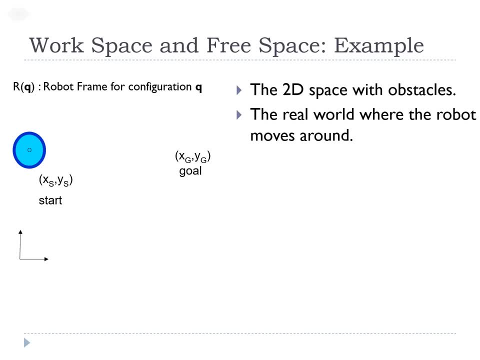 is XGYG. There are many ways to configure a robot. So, for example, if you want to configure a robot, you can configure a robot in which the robot can move from XSYS to XGYG or the goal position. Straight line is one such simple path. So the valid paths will be those paths where the robot 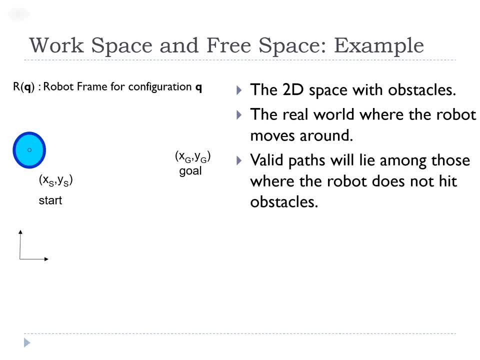 does not hit any obstacle. Here there is no obstacle shown, But think of an obstacle in between. You will definitely consider a path which is not hitting the obstacle. Set of all those configurations for which the robot does not hit any obstacle, you will definitely consider a path which is not hitting the obstacle. 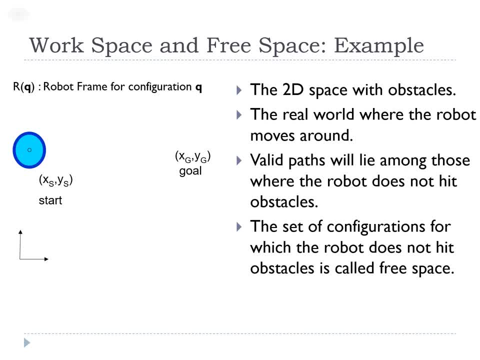 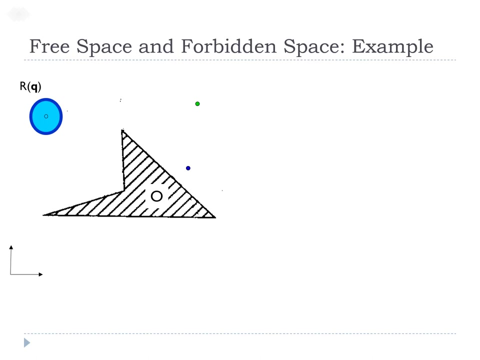 is called a free space. So that is the difference between a free space and the workspace. Let us take an example to understand what is a free space and a forbidden space. In this example you can see that there is a robot R, which is a disk robot. 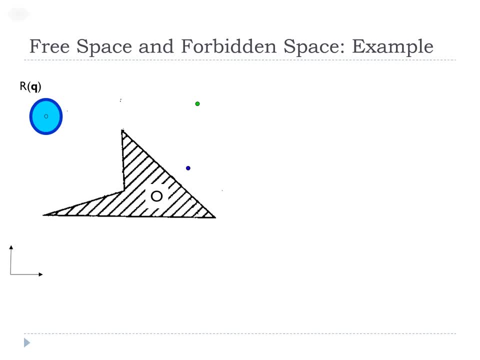 robot at a configuration Q and there is an obstacle O. Now what is a free space? A free space is the collection of all those configurations, so that robot at those configuration does not collide with the obstacle. So what is a forbidden space? in this case, Forbidden space will be. 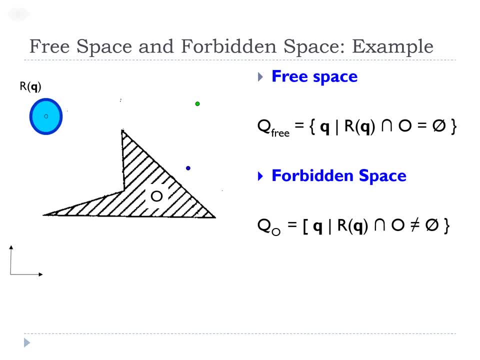 all those configurations of the robot which are having some intersection or collision with the obstacle. So see this position, it is completely free, it is not colliding with the obstacle In this way. all these positions are free configurations. So if we consider this boundary, that on this boundary, the robot, if I consider the center of the robot, the path of the center, 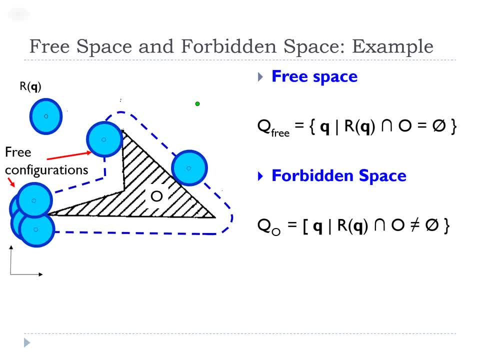 of the robot is shown, which shows that these configurations are all free configurations. If I consider any other configuration like this, shown by red position of the robot, it is a forbidden configuration because it is colliding with the obstacle. Suppose you have to plan a path from. 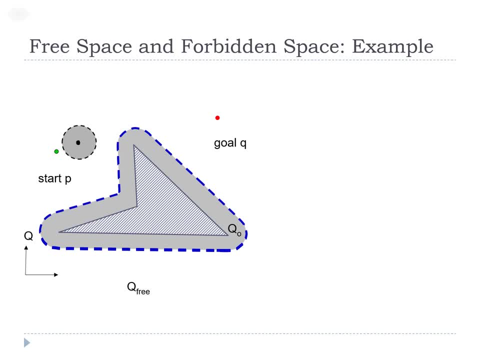 the start, configuration P, shown by green dot, to the goal configuration Q, shown by red dot. What we will be doing? we will be checking all those configurations which are free configuration. So if intersection of P with forbidden configuration Q O is empty, then path is, in Q, free. that means it. 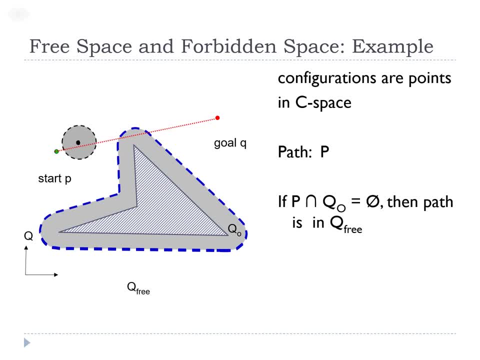 avoids the obstacle. So, if I consider a straight line path, which is very simple path, what will happen at this position? the configuration will not be free or the robot will be colliding with the obstacle. In order to avoid this collision, we construct a different path, which is a piecewise. 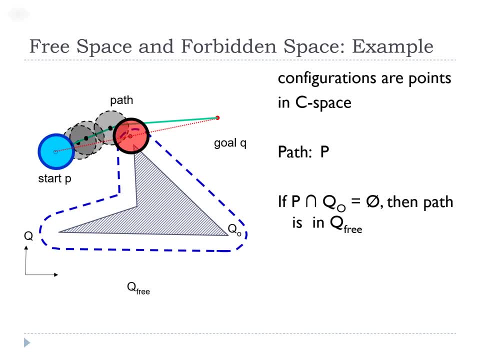 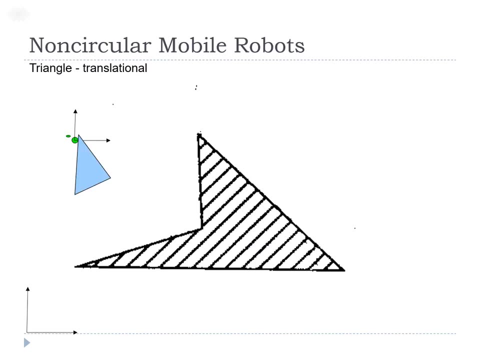 linear path. Now you can see that the robot can move easily with no collision with the obstacle. So this is a path which is in the free space For circular robot. we saw how we can construct Q free or free configuration space by just sliding the robot on the periphery or the boundary of the obstacle. 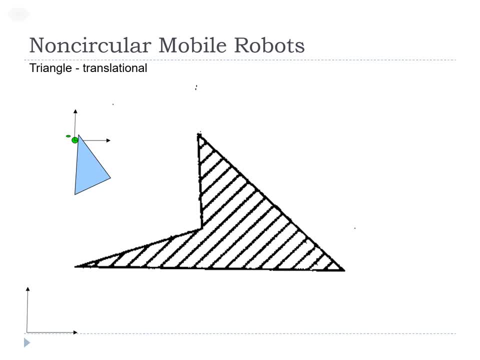 Similarly for a non-circular mobile robot like a triangle shown here. let us see how do we construct. We will do the same thing by sliding the robot throughout the boundary of the obstacle, and here you can see that the edges of the C space obstacle are parallel to. 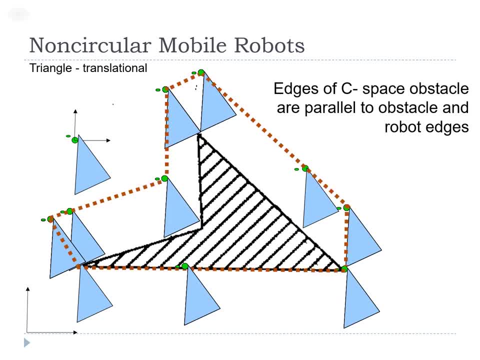 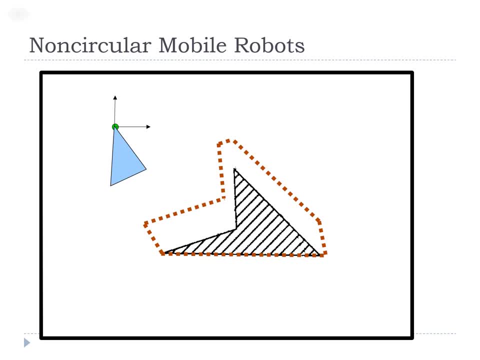 the obstacle and robot edges. So for this triangular robot having only two degrees of freedom of translation in x and y direction, the free configuration space is any position which is beyond this red boundary which is not containing the obstacle, and within this red boundary containing the obstacle, you have the forbidden space. 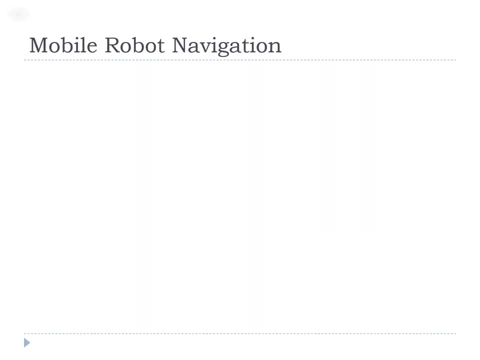 Next, let us discuss what is mobile robot navigation. So navigation is a process of determining or maintaining a course of trajectory to a goal location. It can be any goal, It can be a goal from a one position to another position for a mobile robot, or it can be one configuration to another configuration for a industrial robot. 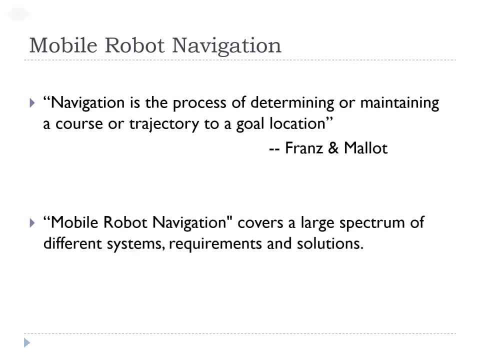 as defined by France and Bernard. So mobile robot navigation covers a large spectrum of different systems, requirements and solution. For example, you have to define the entire workspace, all the geometries and dimensions of every single obstacle that is present. What is the dimension of the? 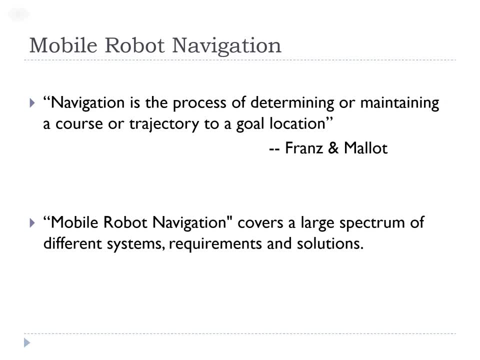 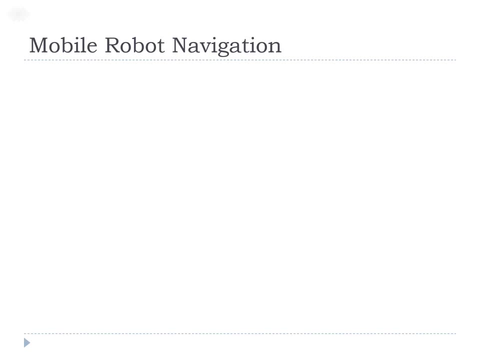 workspace. What are different requirements of the robot? It can be navigation, It can be coverage of area, or it can be picking up an object and placing at some other place. So, accordingly, we have to define these solutions Depending upon different types of tasks. a robot has to perform: navigations. 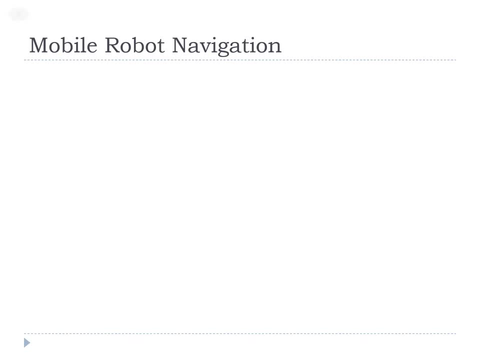 are accordingly defined. These are broadly categorized into four categories. One is global navigation. Global navigation is what is a reality. Suppose you have to start from a one corner of a room to another corner of a room. Robot's determination of where exactly it is at a current point of time and how it. 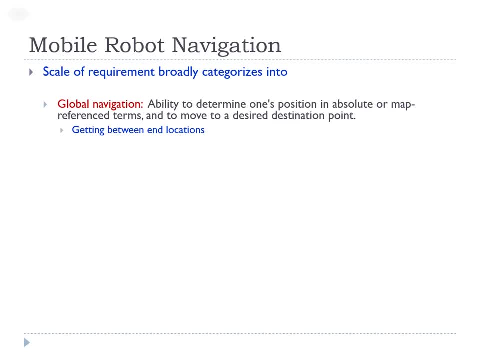 has to reach the destination is what is known as the global navigation. Local navigation, on the other hand, will be the ability to determine one's position related to objects- It can be a stationary object or a moving object in the environment- and to interact with them correctly, so carrying out a task while a look at a location personal. 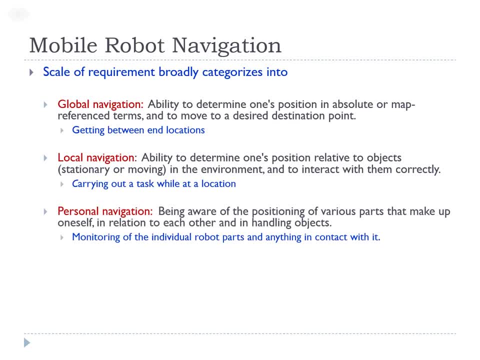 navigation, on the other hand, is being aware of the positioning of various parts that may cut up, make up a robot. it can be different hands of a humanoid robot or legs, so accordingly it has to take a position so that it is able to navigate properly in the environment. 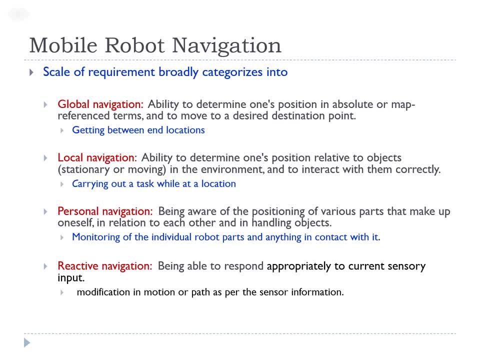 finally, the reactive navigation. it is being able to respond appropriately to current sensory input. so if the sensory input says that a robot, another robot, is coming from the front, then it has to take a different course of action. that is what is known as the reactive navigation. here is an. 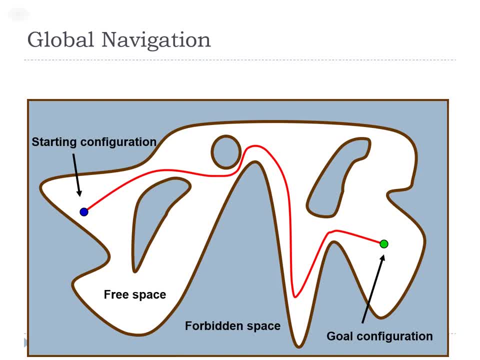 example showing that we have a starting configuration shown by the blue dot, a goal configuration shown by the blue dot, and then we have a starting configuration shown by the blue dot, and then we have a starting configuration shown by the green dot, in the white space, which is a 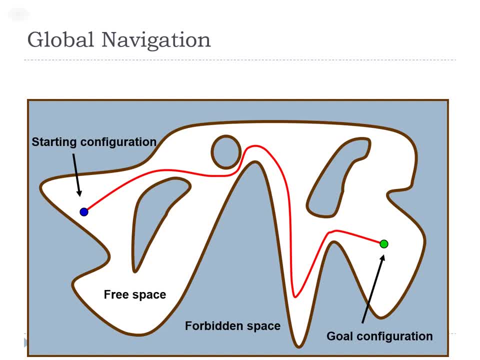 green dot in the white space, which is a free space, and if you have gray space, that is all forbidden space. so that means there are obstacles in that space. accordingly, a red path is shown which is showing how the robot will be globally moving, that is, global navigation. 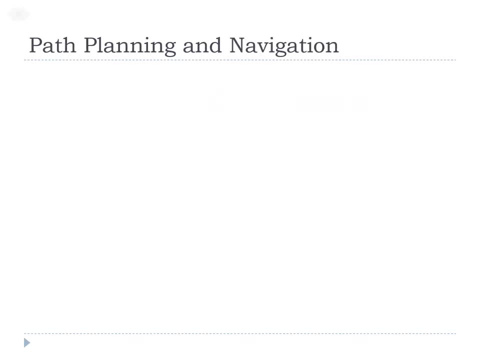 paths, planning and navigation is done in different types of environment. one is known environment where the geometry and topology of each object, including the obstacles in the workspace, is known. such an environment is known as a known environment, as is told you that a room having all furniture. so if this is known a priori to the robot, then this is known as a known environment. a known environment, on the other hand, is an environment in which the environment is adjustableOO. the environment is an environment which is, in our comprend night you can see, drawn as an office spacelegen. so this is how you know that the environment, in the treatment of it, measured, that the robot is Dust release and how the robotic award than this is too, as a known environment. a known environment, on the other. 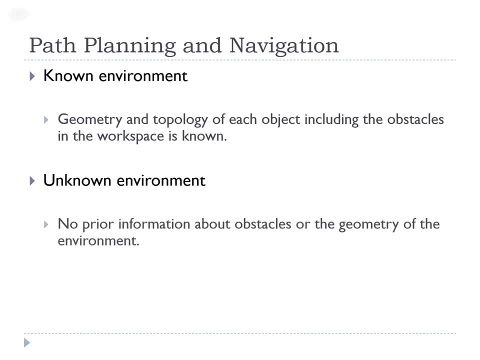 then you ask how it will be used in such a situation. thisGL- I am going to describe the activity involved in this different- to apply this architecture so that this is something that is going to be done in the interactions that we may need né where you don't have any information, or the robot does not have any information about the obstacles. 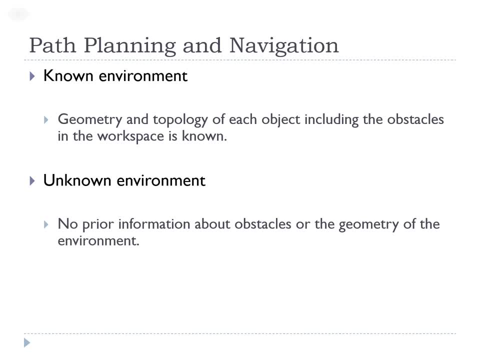 or the geometry of the environment, but it only knows what is the task, that is, what is the starting configuration and the goal configuration. Partially known environment are those environment where, through the sensory inputs, the robot is able to know locally the environment. Now you must have understood what are the basics of path planning. First thing, 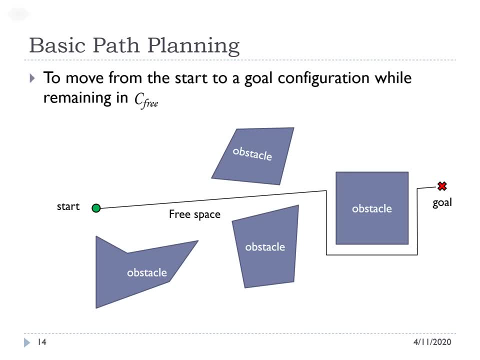 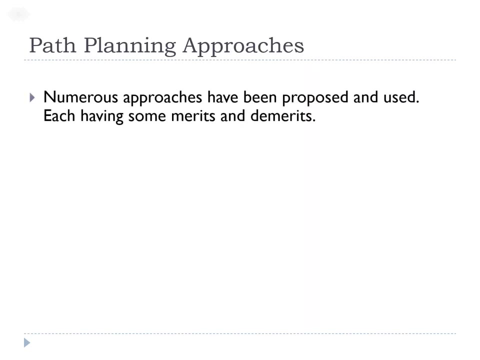 to move from the start to a goal configuration while remaining in the free configuration space. Here is an example showing the start location and the goal location and also the path that shows that within the free space one has to move. Numerous path planning approaches have been. 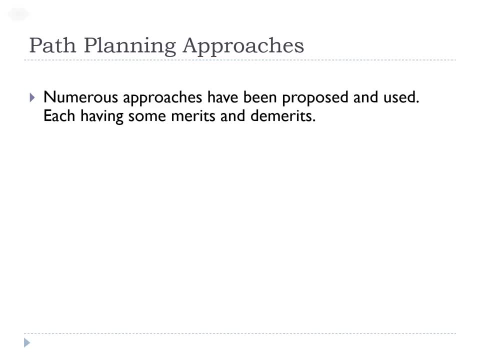 proposed over the years. Each is having some merits and demerits. Depending on robotic task, one has to move from the start to a goal configuration while remaining in the free configuration space. These approaches are applied, For example, for unknown environment. there are some. 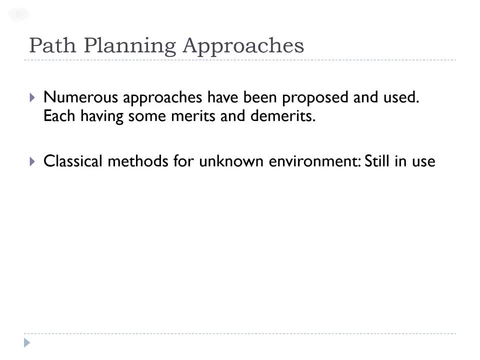 classical methods which are still in use. They have been studied thoroughly and have been refined by various researchers. Bug one, bug, two, tangent bug are some of these classical methods. Let us see how they work. So the basic principle of working is like this: You have a start position and a 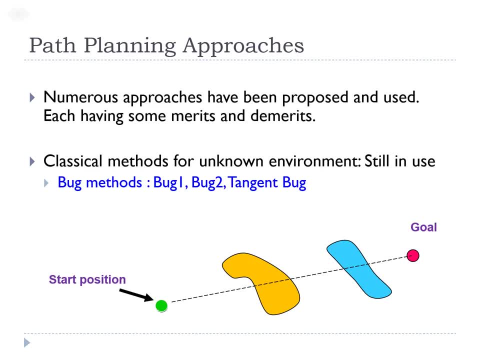 goal position. That is the only thing known to the robot. There is no information about the environment. So it creates an imaginary line between the start and goal position and it follows that straight line until and unless it finds or senses that there is an obstacle in between. So 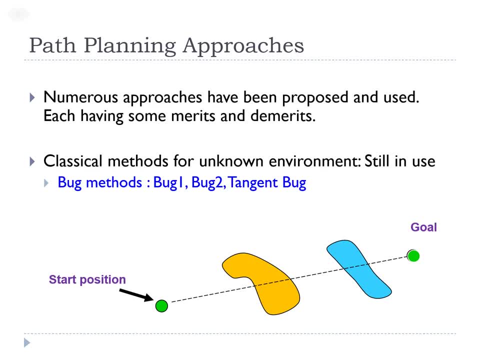 here there are two obstacles that are shown, and the robot will keep on moving until it receives the information that there is an obstacle. Accordingly, it will change its course of action Depending on the strategies followed. bug one, bug two and tangent bug are defined. Online or single stage methods are used when 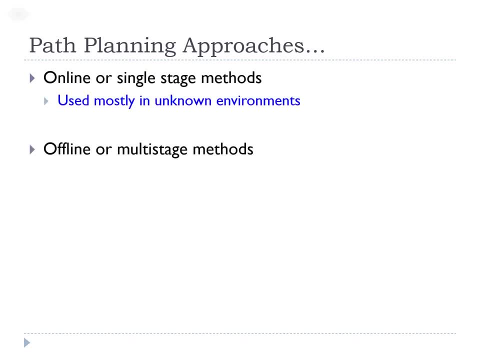 you have no information about the environment, and offline or multi-stage methods are mostly used in cases or applications where the geometry of the environment and obstacles are known beforehand. We begin our discussion with bug navigation algorithm, As I told you that they do not require a priori knowledge of the environment, So we are going to start with. 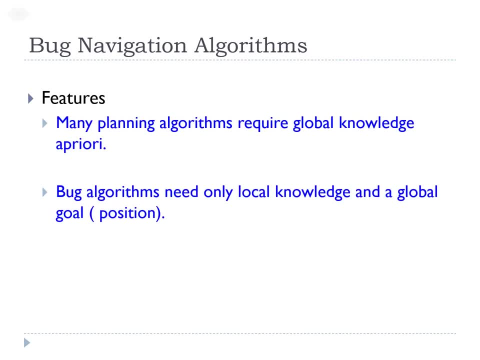 bug navigation algorithm. They only need to know what is the current position of the robot and what is the goal position. These are very simple to implement. Their behavior is simple And bug one and bug two algorithm deal with tactile sensing or touch sensing, whereas tangent bug algorithm 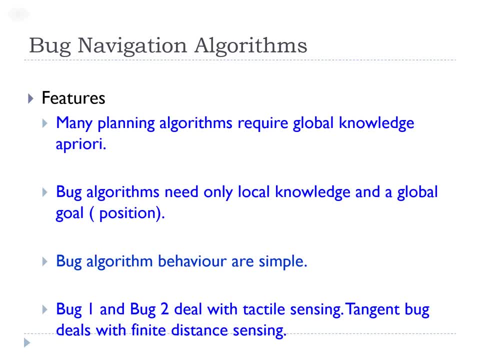 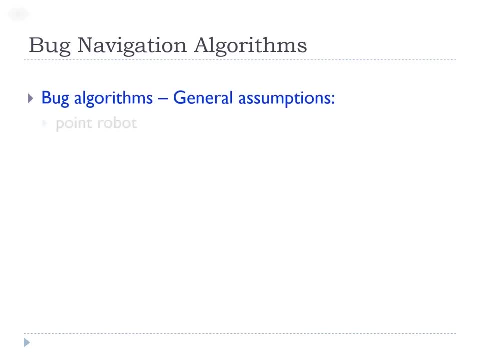 deals with finite distance sensing where you have ultrasonic or the optical camera or any kind of sensor available. Bug algorithms make some general assumptions. They are not just about the distance. First of all, that the robot is a point robot. Remember that configuration space is so. 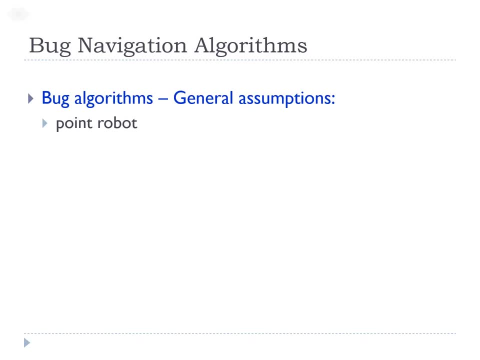 defined that the robot can be considered as a point robot, So that's nothing to worry about. Secondly, known goal location. It knows its current position and also the goal location, And the assumption is that there are only finite number of bounded obstacles, which is also very simple to. 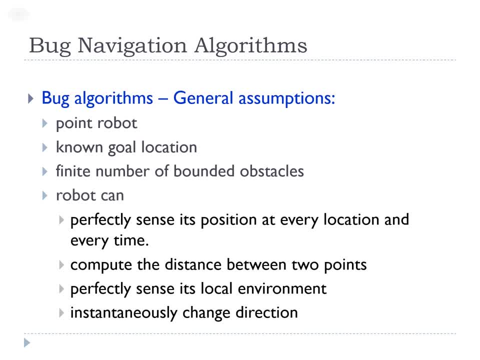 assume Then robot is a point robot. It knows its current position and also the goal location, What can perfectly sense its position at each location and every time. That is very important. It can compute the distance between two points. That means the current position. 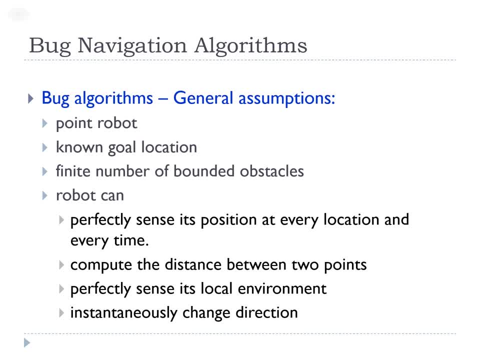 and the goal position or from a position to the goal location, And also perfectly sense its local environment in terms of touch sensing or using the distance sensing, And then instantaneously it can change direction. These are basic assumptions that we make about bug algorithm, And we will see later that how these algorithms are applied to a robot. 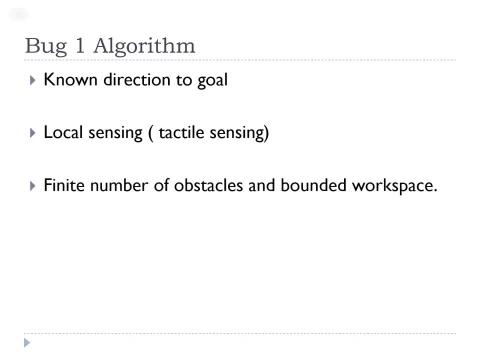 So we first discuss bug one algorithm. As I told, known direction to goal, local sensing, that is, tactile sensing, finite number of obstacles and bounded environment. Bug one algorithm is very simple. Think of a straight line passing from the current position of the robot to the goal location. That is, starting position to the goal location. Then the robot moves. 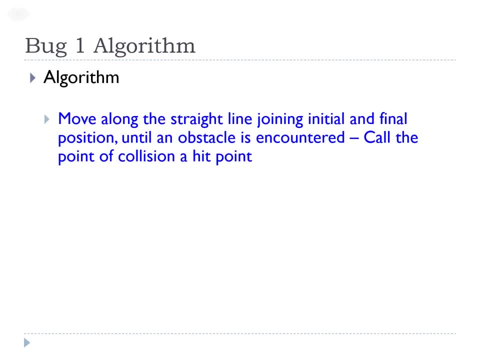 along that straight line and until an obstacle is encountered, it keeps on moving. Once the obstacle is encountered, it calls that point as a hit point. Now, from that position, the hit point, the robot starts moving along the boundary or the periphery of the obstacle And from each point, 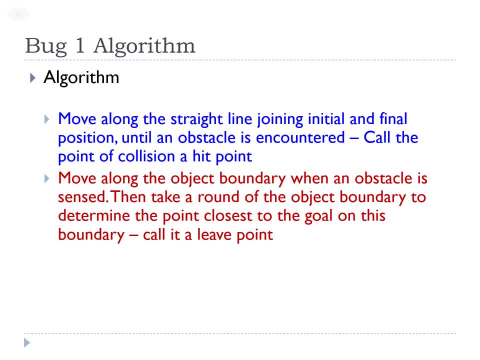 on the boundary of the obstacle. it determines the distance of the current point to the goal. This is the goal location and it finds out a point which is the closest to the goal on the boundary of the obstacle. Call it as a leaf point. Exit from this leaf point toward the goal along the straight line. 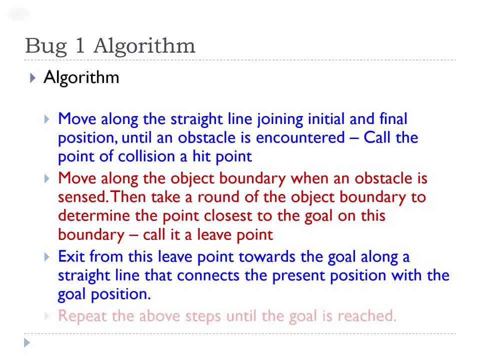 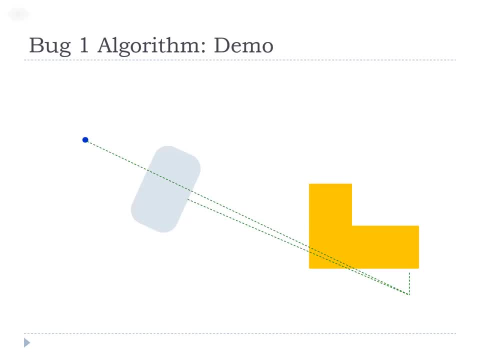 that connects the present position with the goal location and this process is repeated until the goal is reached. And here comes a demo of Bhagwan algorithm. This point robot moves along a straight line to the goal. Then it finds out the obstacle, It moves around the boundary of the obstacle and 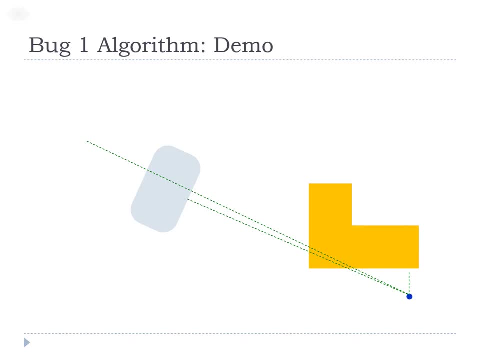 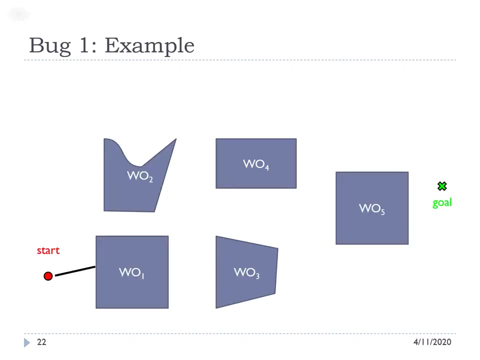 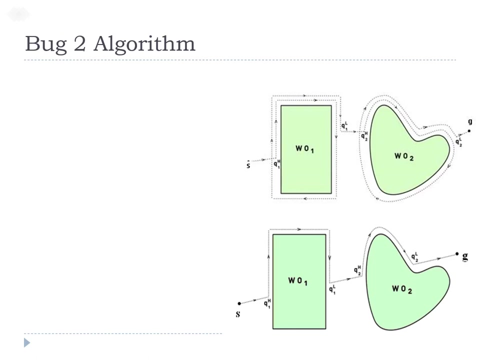 finds out the closest point that is closest to the goal, and then it leaves the obstacle boundary. from that point You can see another demo. Bhaktu algorithm is similar to Bhagwan algorithm, except that it adopts a greedy approach. So it moves along the same straight line, joining the initial. 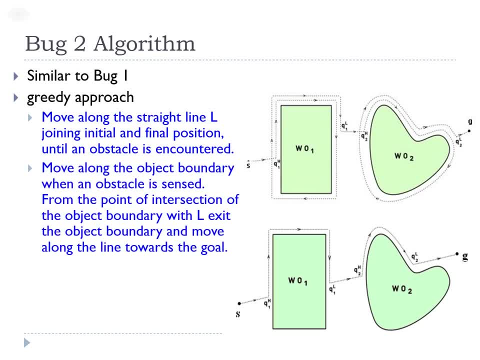 and the final position Until an obstacle is encountered. But when the obstacle is sensed it will move along the obstacle boundary, only to find out the point of intersection of the original line with the obstacle boundary, as you can see in the bottom figure. So bottom figure is for Bhaktu algorithm. 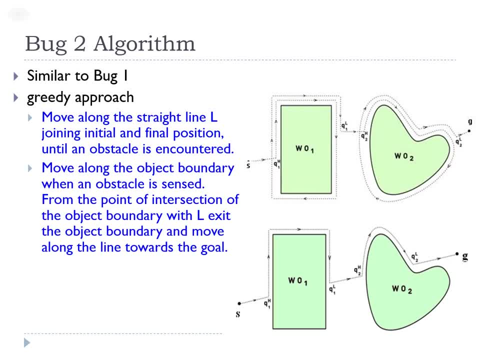 and the top figure is for Bhagwan algorithm. You can see that Bhagwan algorithm takes an exhaustive search to find out the leaf point which is closest to the goal point, Whereas here in Bhaktu algorithm, it is adopting a greedy approach As soon as it senses the point. 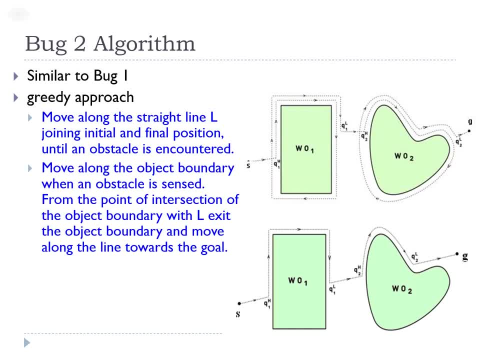 of intersection of the original line with the obstacle boundary, it will leave the obstacle boundary. If an obstacle is sense, again the same process is repeated. So until the goal is reached, the same process is repeated again and again. One behavior is: move along a straight line. the other behavior is follow the path of the destination. In all the 쓰는 two types of behavior: the upper one is developed, the upper two areeloved and the lower one is lessるence elenc больше escuched. 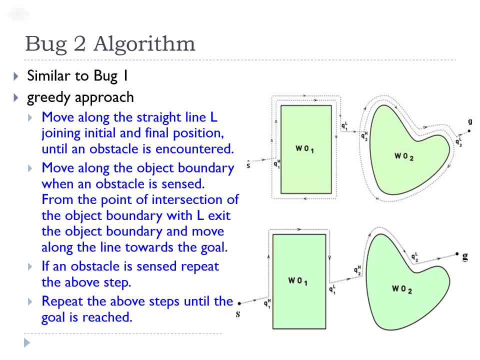 He flies up, walks, leaves three places and moves in a straight line but runs in another direction. As your notice, it has a very vigorous form to follow the entire process. If you plan it, then mom is high by follow the obstacle boundary. in bug1 algorithm and bug2 algorithm there is a small difference. 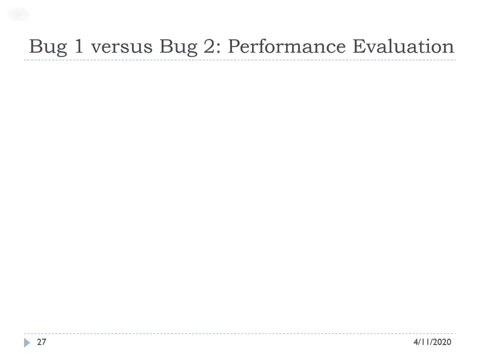 as you can see, bug1 versus bug2- there are several performance evaluation studies done on different scenarios and bug1, you know it uses an exhaustive search because it considers all leaf points before leaving the obstacle, whereas bug2 uses a greedy search, it takes the first leaf point, that is. 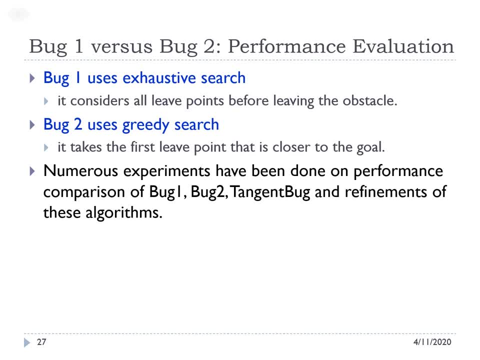 closer to the goal. numerous experiments have been done on performance comparison of bug1, bug2, tangent, bug and several refinements of these algorithms, but it has been found that on different scenarios each of these algorithms perform better in terms of path length or computational time or memory requirement, so we cannot say that any one of these algorithms is doing well. 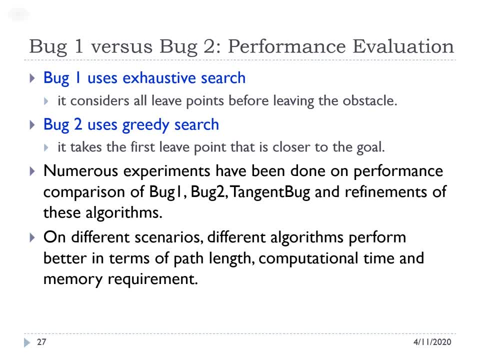 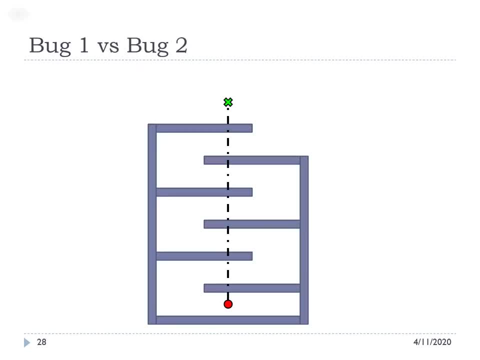 you must have seen that bug1 is using exhaustive search, so the time taken might be very high, but it depends on scenario, as we shall see. so finally, this interesting exercise for you to check the performance of bug1 and bug2, compare their performance. here, green check is the starting. 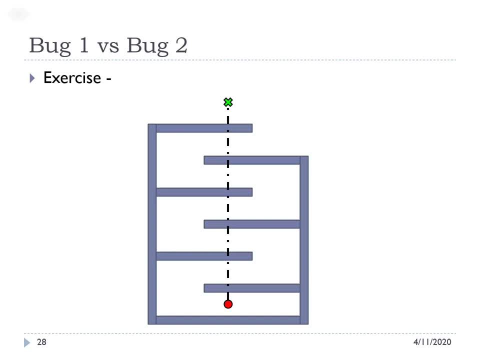 position. red dot is the final position or the end position. you have to find out the path using bug1 and then using bug2. the only limitation here is that the robot moves left as soon as it senses an obstacle, boundary or obstacle. stay tuned. we will be discussing more on tangent bug algorithm in our next session.